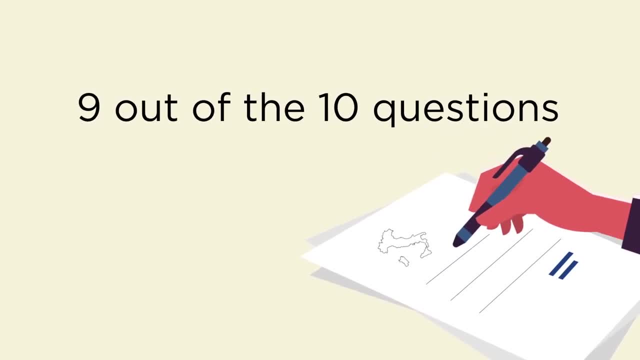 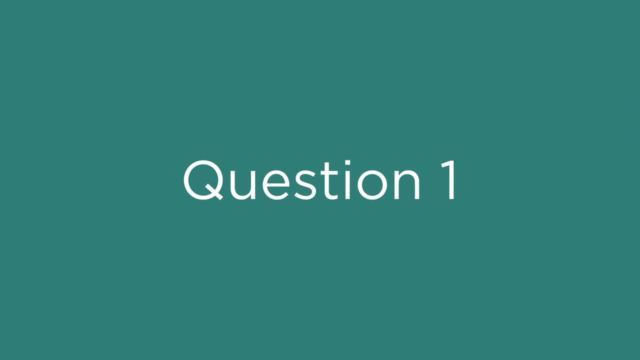 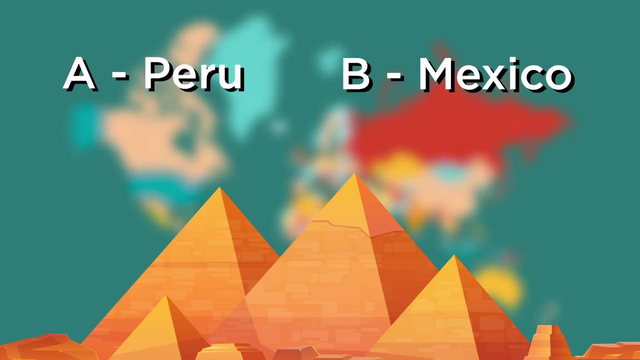 correctly, so make sure you keep track of your score. You will be graded at the end of the video. Are you ready? It's time to begin. Question number one: Where would you find the Great Pyramid of Giza? Is it A Peru, B Mexico, C Egypt or D Morocco? 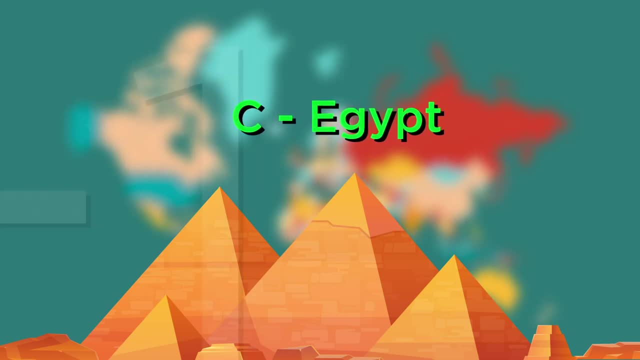 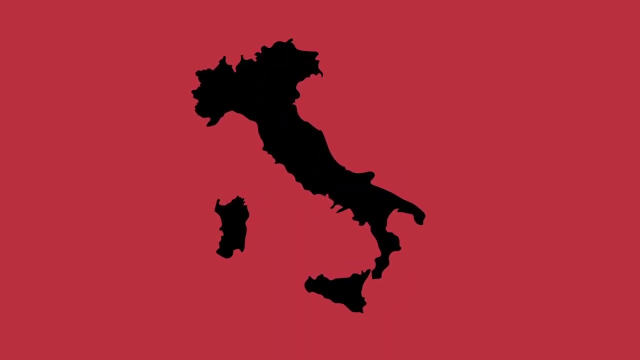 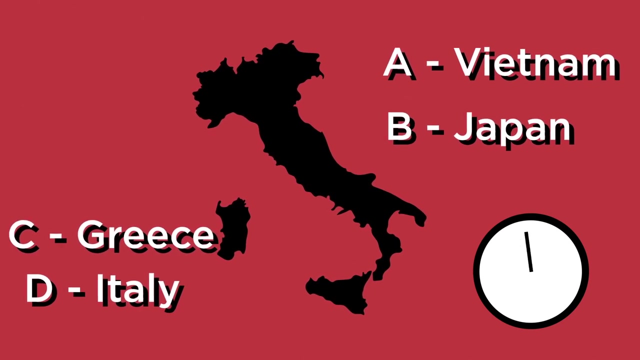 The answer is C- Egypt. If you got it right, give yourself a point. Question number two: What country is this? Is it A Vietnam, B Japan, C Greece or D Italy? The answer is D Italy. If you answered correctly, give yourself a point. 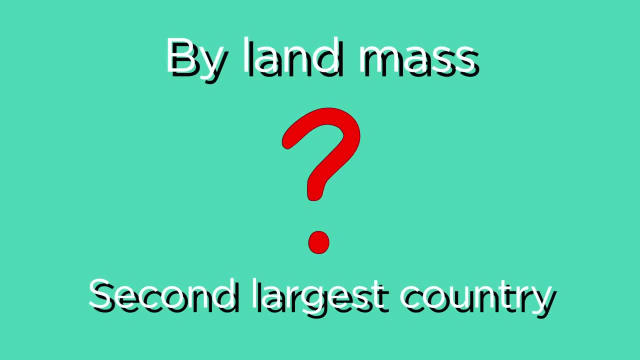 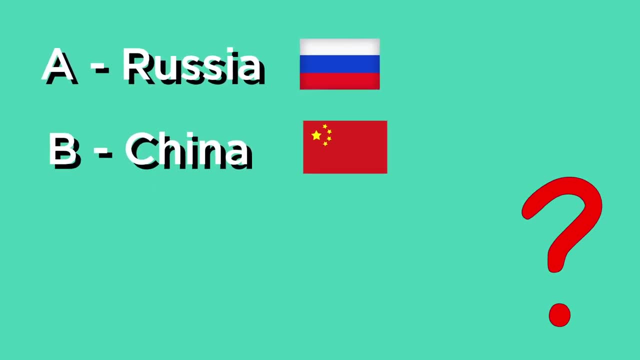 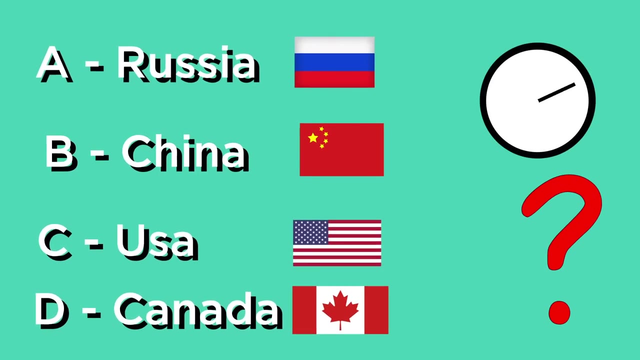 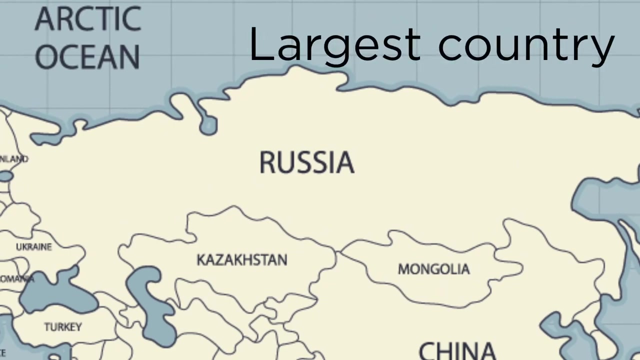 Question three: By landmass, what is the second largest country in the world? Is it A- Russia, B- China, C, USA or D- Canada? Russia is the largest country on Earth, covering over 17 million square miles. 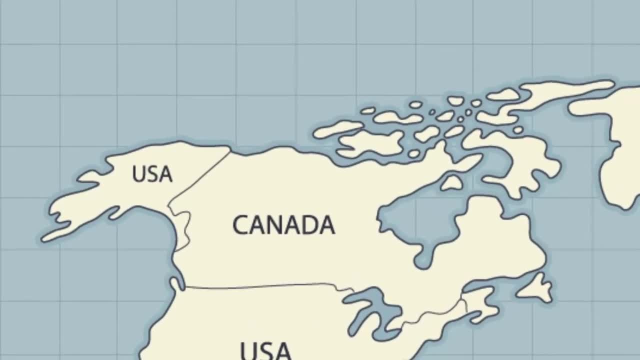 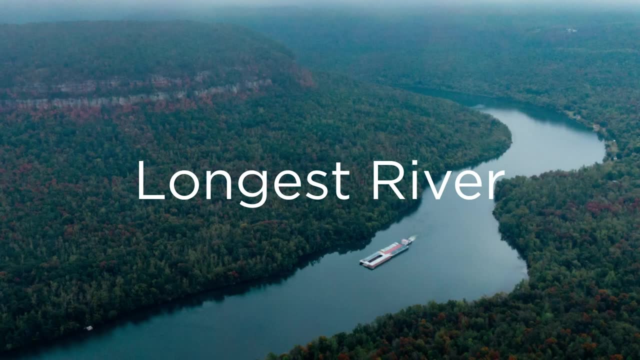 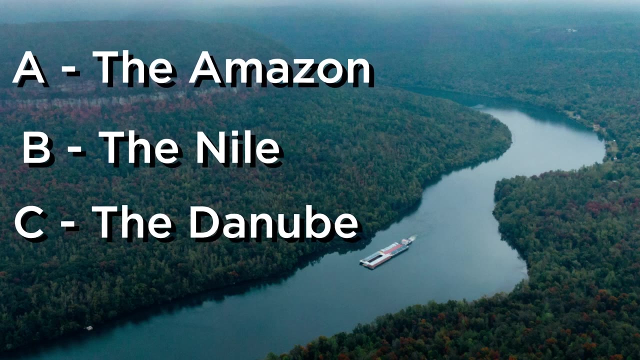 but the second largest is Canada. So if you answered D, give yourself a point. Question number four: What is the world's longest river? Is it A- The Amazon, B The Nile, C The Danube or D- The Mississippi? 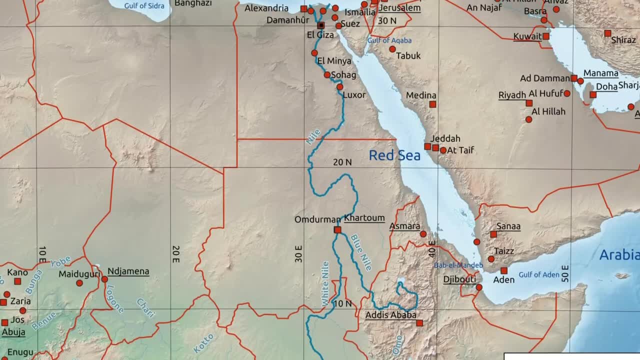 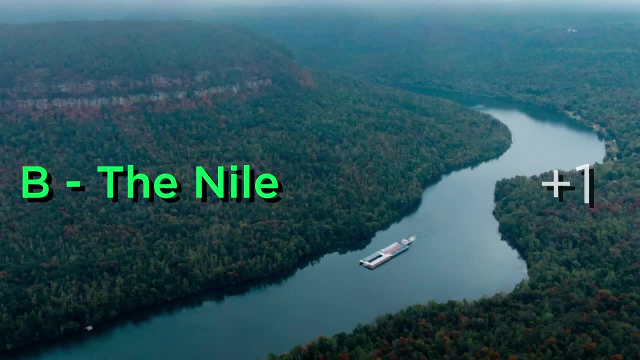 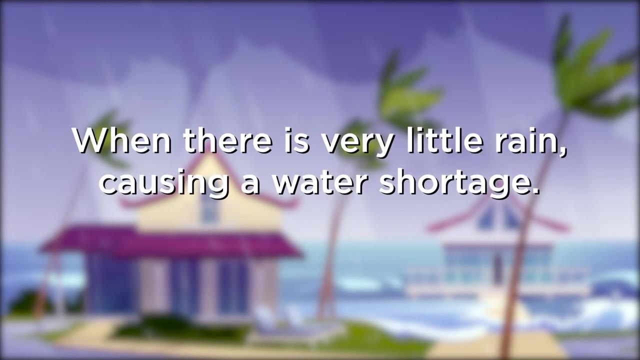 The answer is B: The River Nile, which stretches over 6,000 kilometers across northeastern Africa. If you answered B, give yourself a point. Question five: When there is very little rain causing a water shortage, this is called what? A- A flood, B- Pollution. 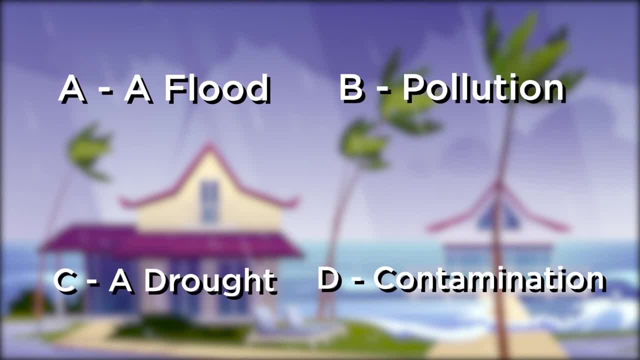 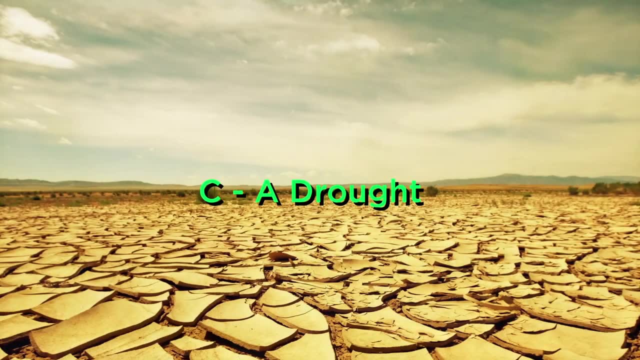 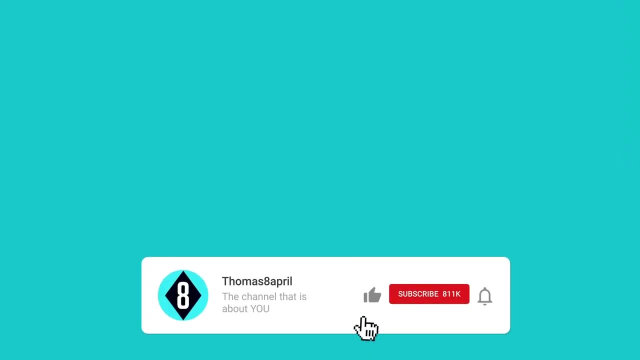 C A drought or D Contamination. The answer is C A- drought. If you got it right, take a point Well done. You've just passed the halfway point, so give the video a quick, like It might give you good luck. Time for question six. What is the largest desert in Africa? Is it A- The Kalahari, B- The Sahara or C- The Sahara? What is the largest desert in Africa? What is the largest desert in Africa? What is the largest desert in Africa?